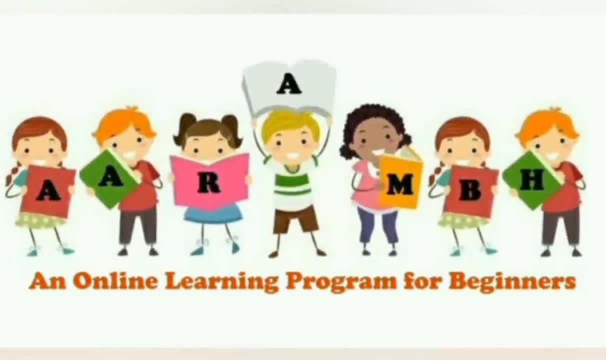 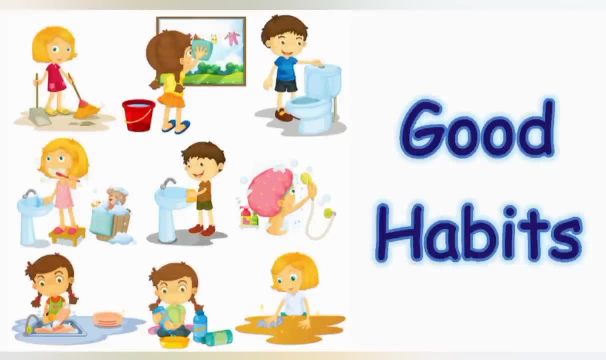 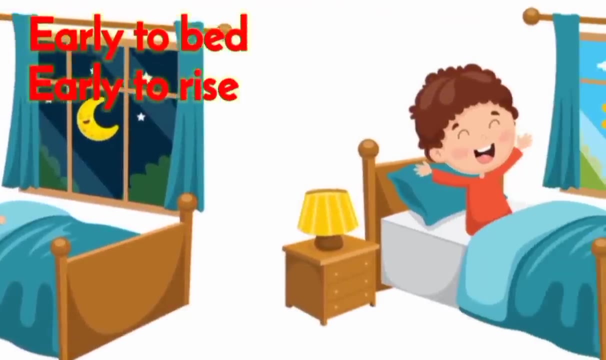 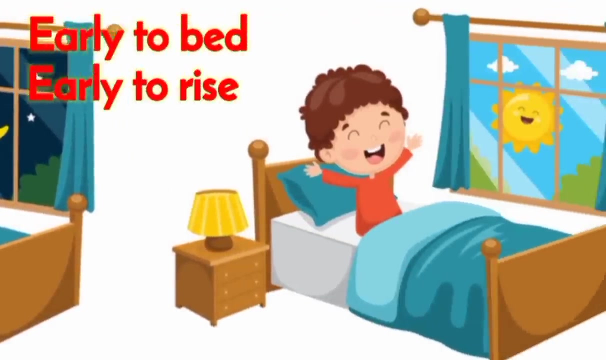 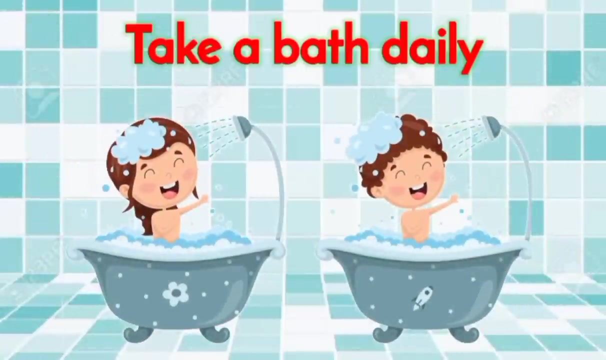 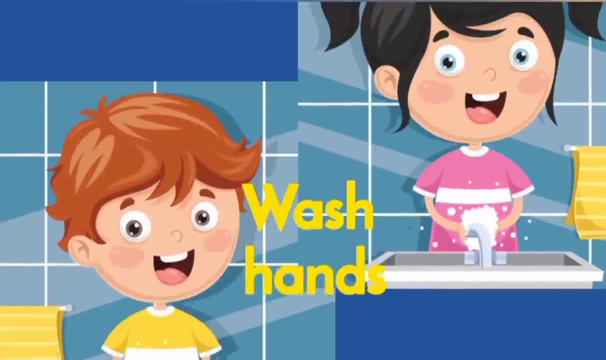 Good Habits, Personal Hygiene and Fitness. Early to bed, early to rise. We should sleep early and wake up early in the morning. to stay healthy and fit, Take a bath daily. Brush your teeth twice a day. We must wash our hands before and after every meal. 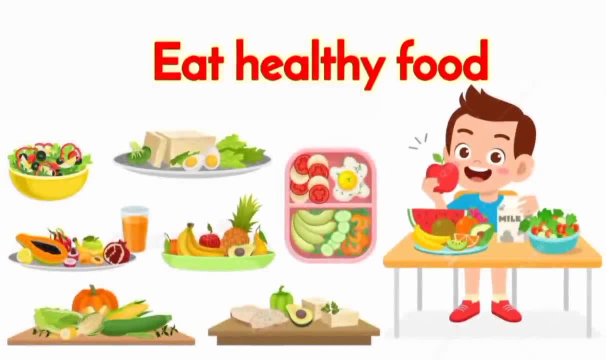 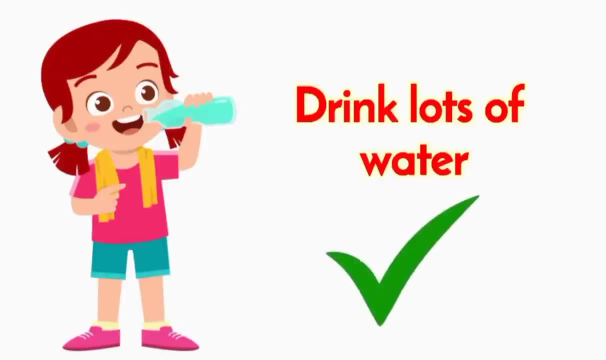 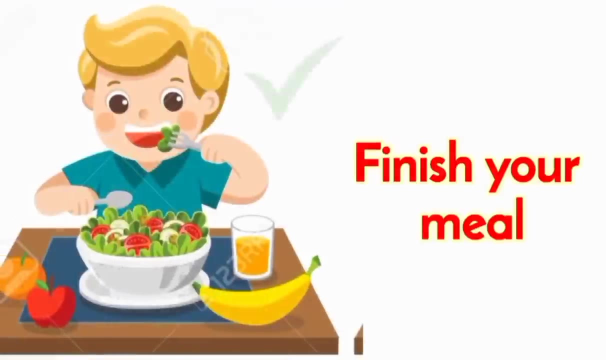 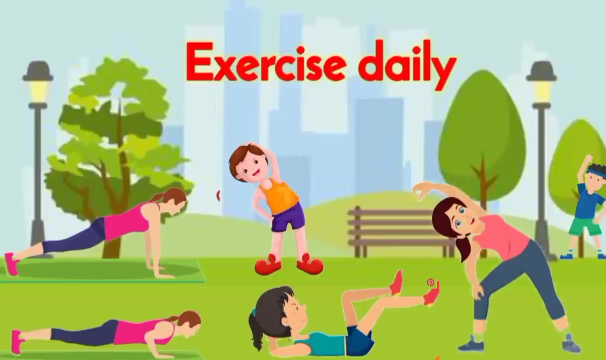 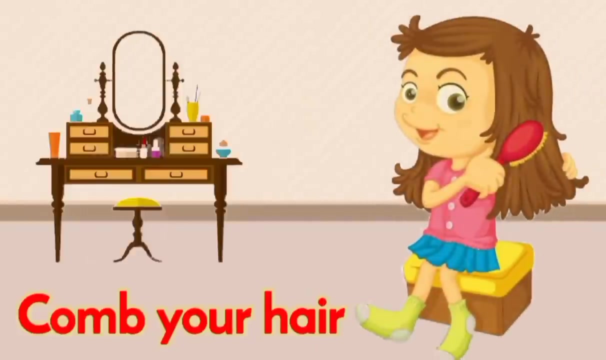 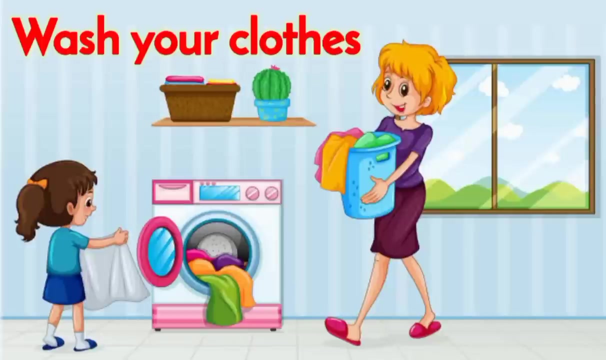 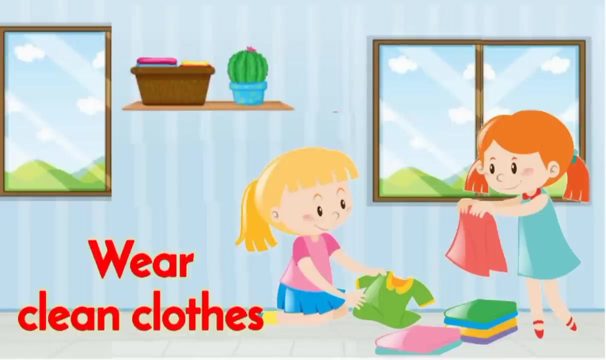 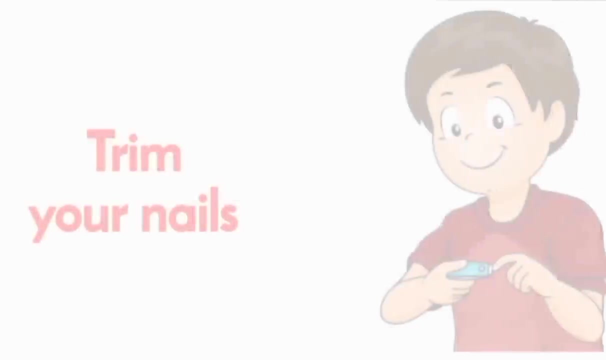 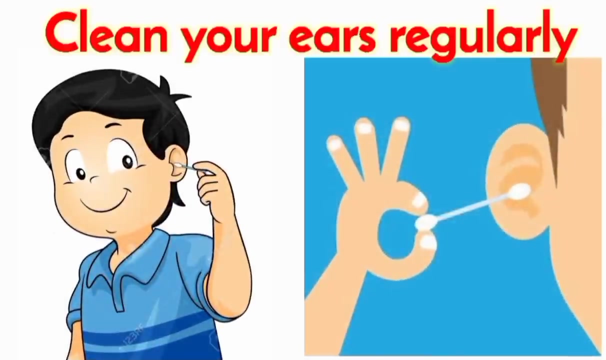 Eat healthy food full of vitamins and minerals. Drink lots of water. Always finish your meal. Exercise daily, Comb your hair twice a day. We must wash our clothes regularly, Iron them And wear Clean clothes. Trim your nails regularly. Clean your ears regularly. 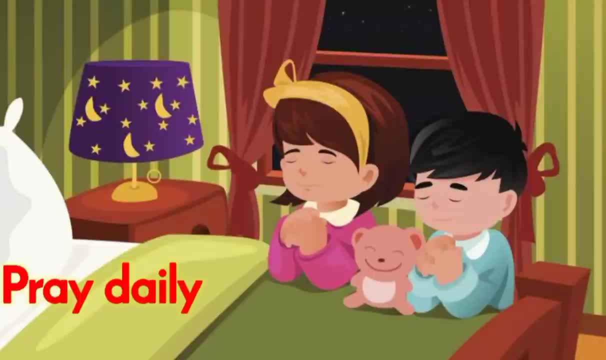 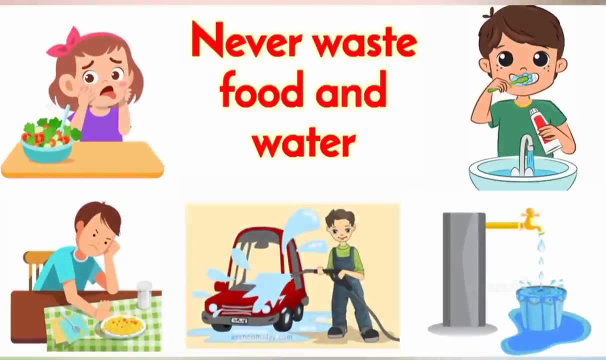 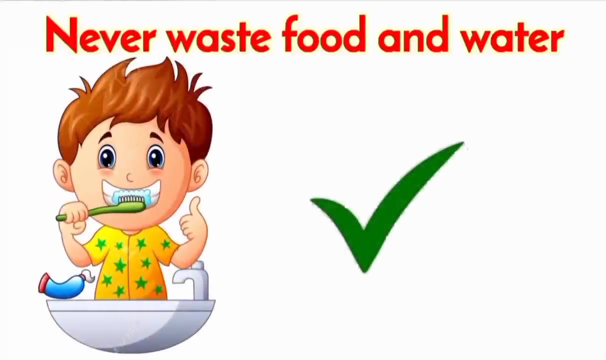 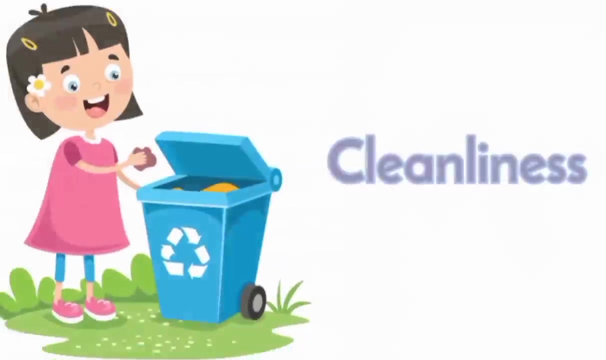 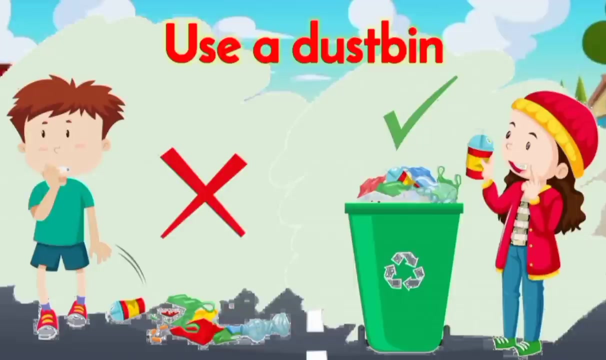 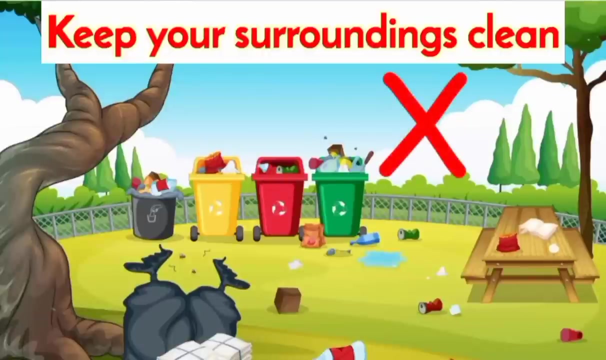 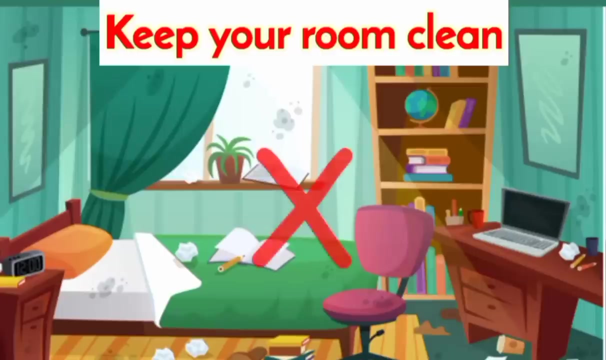 Pray daily In the morning and before going to bed. We should never sleep. Never waste food and water. We should close the tap after use. Finish your food Cleanliness. Throw the garbage in the dustbin. Keep your surroundings clean. 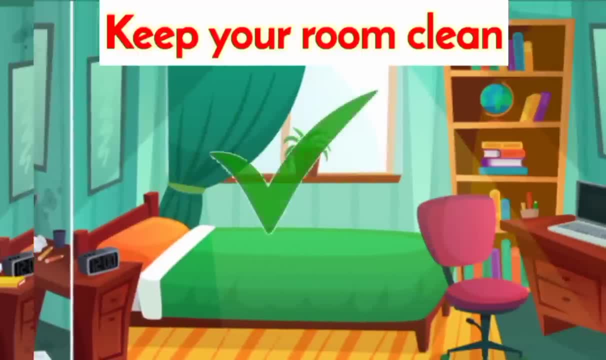 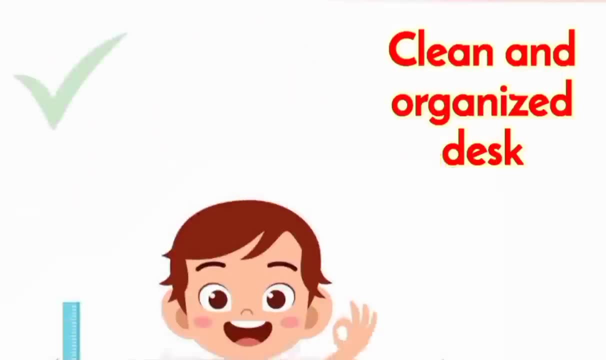